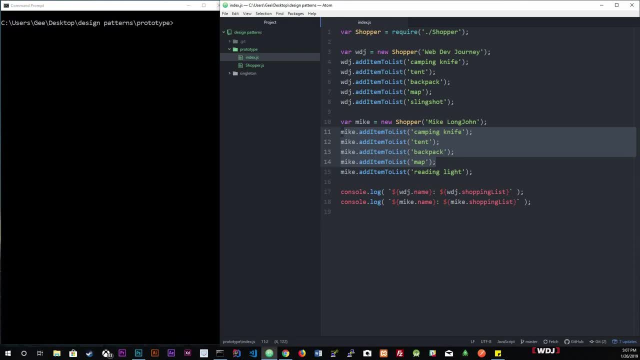 are going camping and it's kind of you probably, uh, we do. we both need a camping knife, tent, backpack and map, just in case one gets lost. we're gonna go with camping knife, tent, backpack and map, just in case one gets lost. we're gonna go with camping knife, tent, backpack and map, just in case one gets lost. 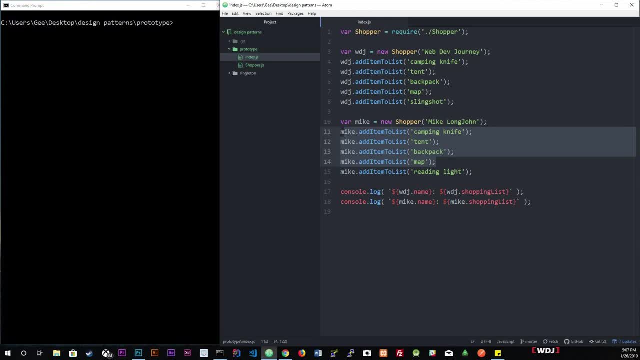 well, at least they have their own map, their own backpack, their own tent and camping knife. but it would be better if we didn't have to actually go out and start grabbing this stuff. you know, it'll be better if someone already had those things for us, so that way we just grab them. 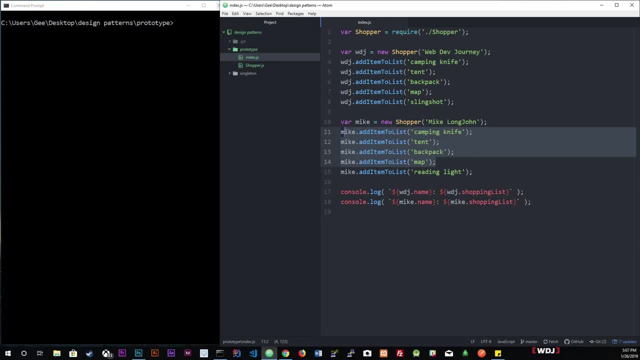 and then just add our own items. you know, we just bring our own items and just go to this person and say, hey, we need these things, and just pay him instead of going out and doing the shopping- our all of ourselves. so that's what we're going to be doing right now. we're actually going to create 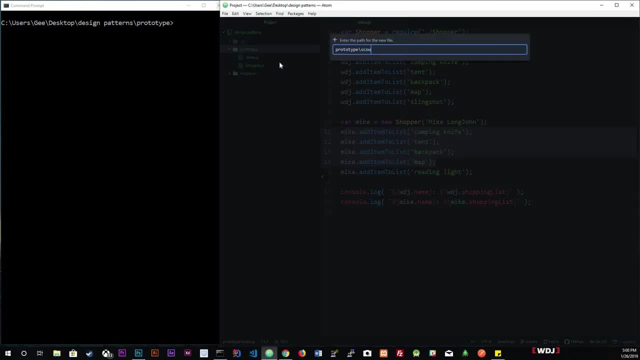 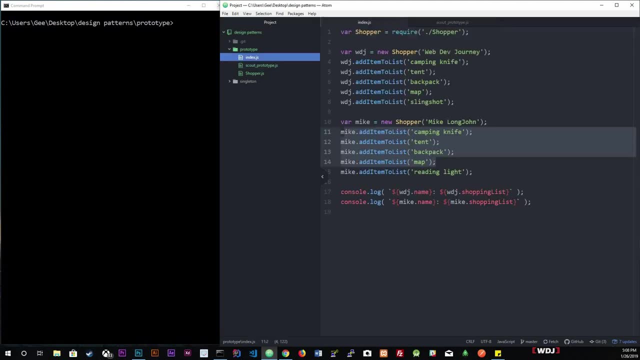 a profile called well, scout, underscore, prototype dot js. and here we're actually going to give this scout. i'm going to copy this, i'm going to call this scout. we're not going to give it a name, we're going to give this scout the- i'm going to say the redundant kind of things that everybody 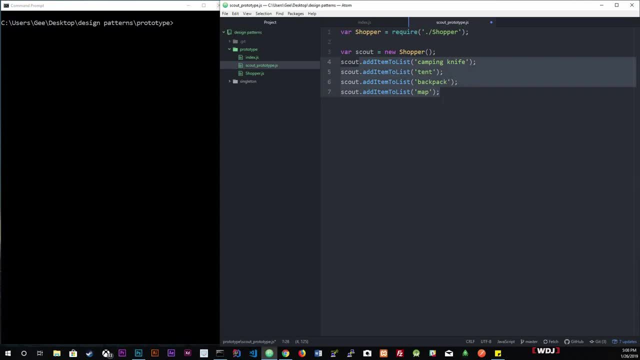 needs. so now this scout is always going to have the camping knife, tent, backpack and map. so we will just ask the scout: hey, we need these things, just give it to us, so that way we don't have to keep on, uh, looking for these things. so we got this scout right here back in index. well, obviously we don't need this and we're 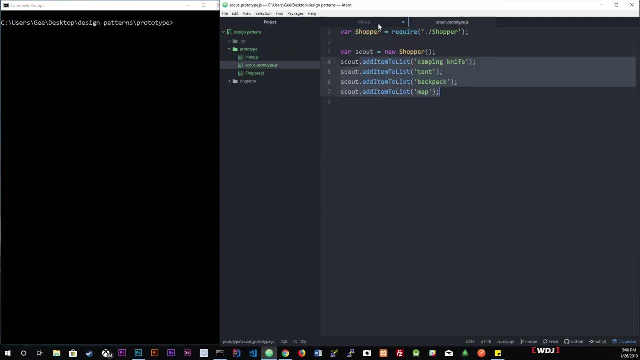 not creating a new instance of shopper, since scout already does that for us. what we're going to be doing is using scout, so i'm going to do- i'm going to require scout, scout underscore prototype. i hope. i hope i spelt that right and we're not going to be creating a new shopper, ratchet. 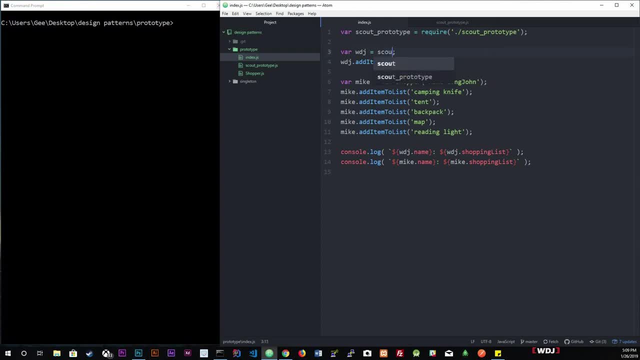 just going to be cloning this scout, so scout, dot clone, and this needs a name. wdj does need a name, so dot name. it's going to equal web dev journey and we're going to do the same thing for the got for Mike. we need to get rid of these things. redundant kind of stuff, just give. 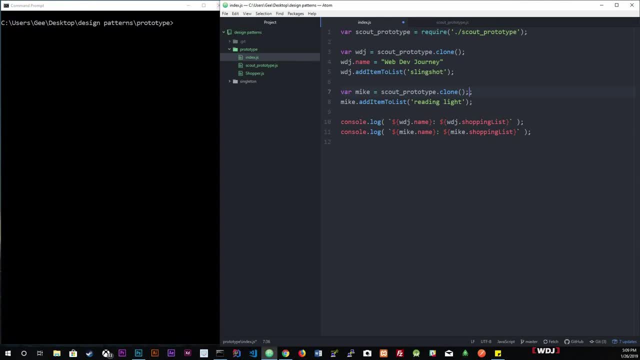 him the Scout, or he's gonna ask out to give him the the things that he needs. so Mike dot name is going to equal Mike long John silver, just like that. all right. so the only thing I'm bringing in the slingshot and the only thing he's- 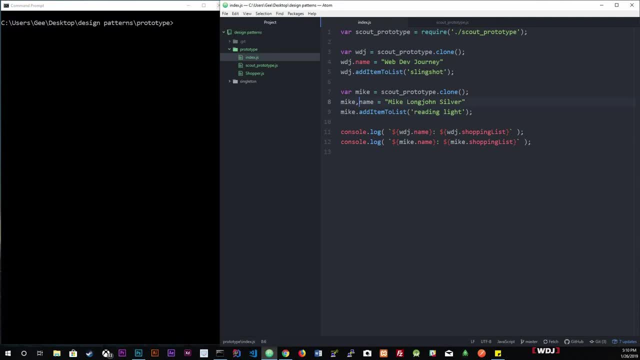 bringing in the reading light and the Scout is gonna provide us with the redundant stuff- it's not really redundant, but the actual necessary things that we need. so before we actually run this, we do need to create our clone method. we don't have it, and before we do that- I think I forgot, yeah. 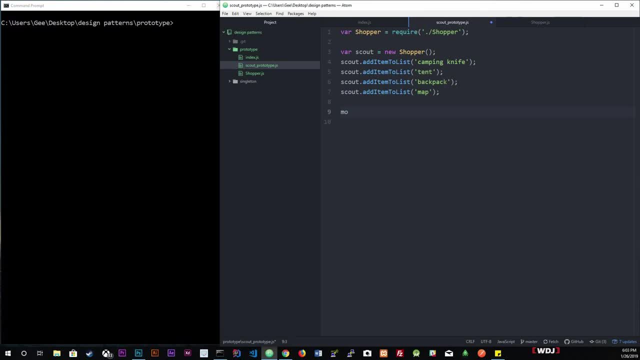 I forgot to export our Scout. so module dot exports equals Scout. all right, now, inside a shopper, we're gonna be creating our clone method- clone- and this part is going to confuse a lot of people. this is where people actually get confused. so this first bit, I'm actually try to write, I'm gonna write. 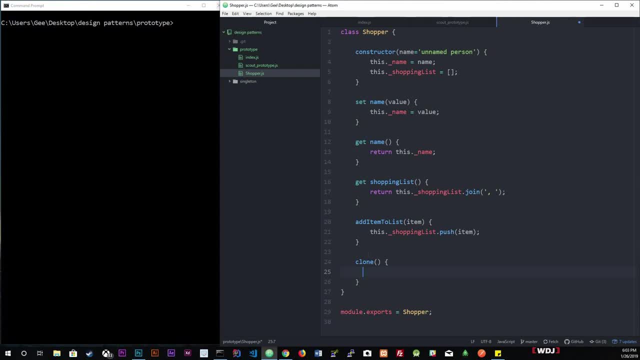 it out and explain somewhat what I'm trying to do and then, once I write it all out, I'm going to explain it. so right now, we're gonna be copying this structure, this shopper structure, over the current instance that we're getting it from. so the current instance is the Scout instant and we're copying the structure. 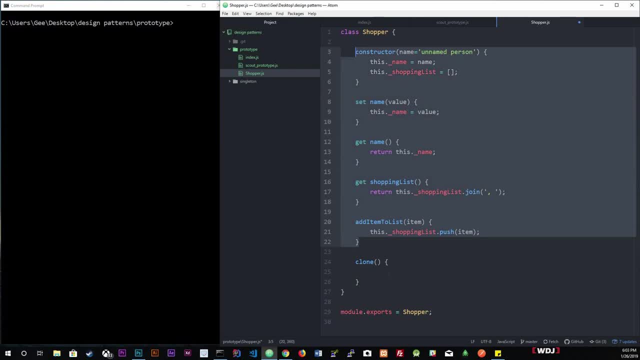 that the Scout has, which is this: so we're gonna call: we're gonna create a variable called proto equals our object dot get proto-type of this. so this line actually grabs the other person's original code and it, like said, I'm gonna the uh, current objects, i mean the current instance structure. now we're going to be creating an object. 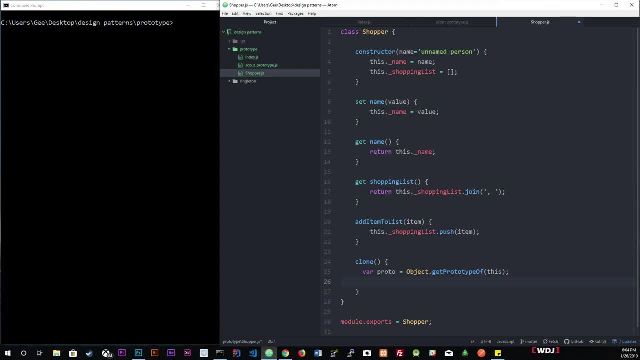 with this structure placed inside of it. so of our clone is going to equal object dot create. we're going to be creating an object and we're going to be sticking this proto, the structure of the object or the structure, the structure. we're going to just give this to the clone now. 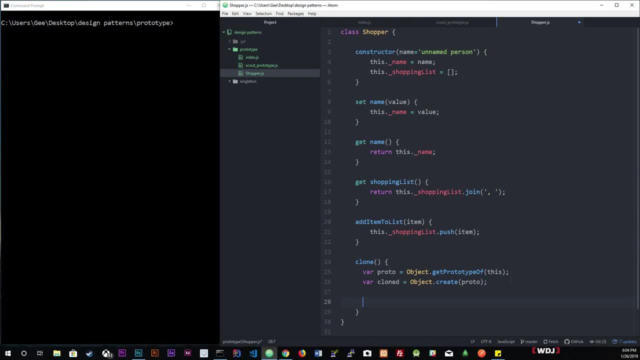 now we are going to. now we do need to get the um, the current values of this- so cloned and we're going to just give it to cloned. so cloned dot underscore name is going to equal this dot underscore name and we do need to do it for shopping list as well. 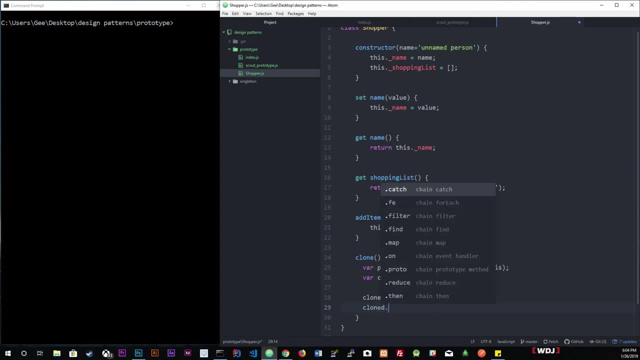 so down here, cloned dot underscore shopping list is going to equal an array or, oops, an array. i'm going to use a spread operator and then this dot shop underscore shopping list. okay, let me explain what's going on right here. so let me actually make this bigger so i can. 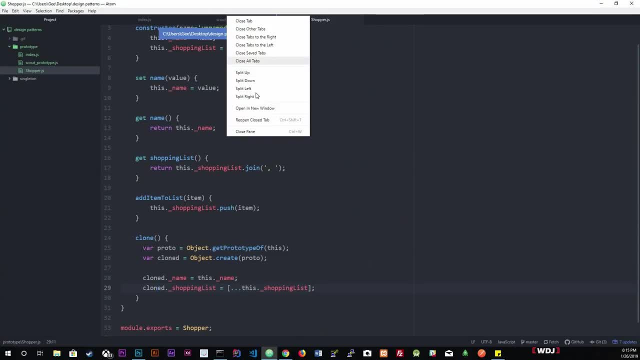 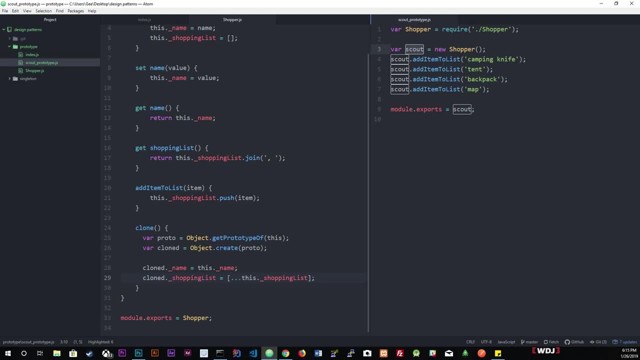 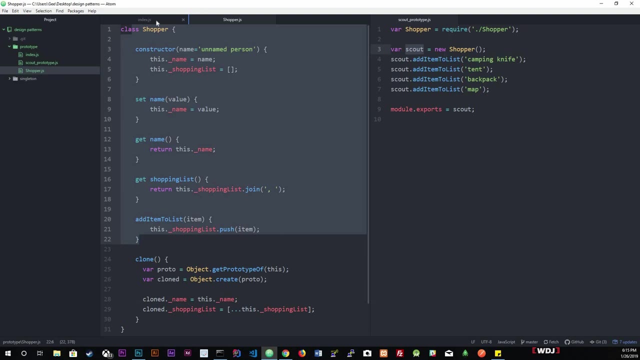 explain it better and i'm actually going to split this to the right. all right, and this is a scout prototype. so over here we have an instance of this shopper class. okay, we have an instance of the shopper class now in indexjs. we're using it, we're cloning it, okay. 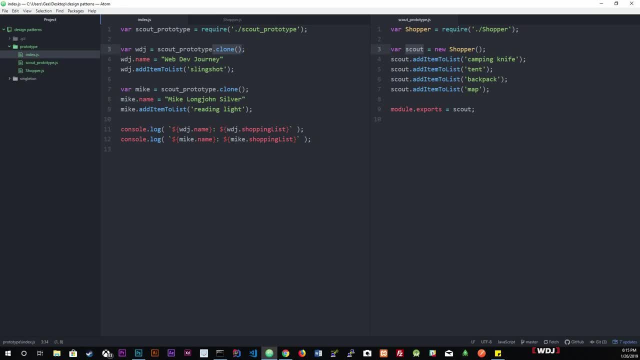 meaning that we don't want to be creating new instances, obviously for the same things. so this is why we clone it. but this scout already has a class stuck to it. it already has is using it. the scout is using a class which is over here. when we clone it, we want to be using the same class. 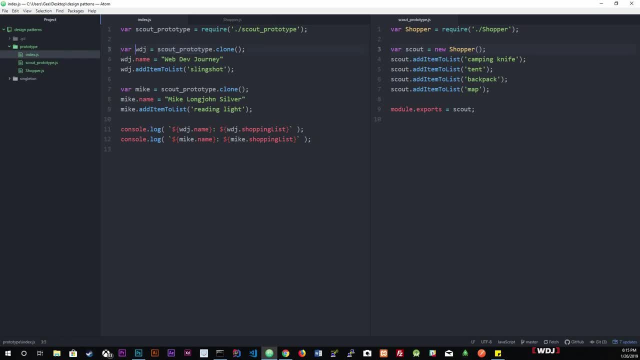 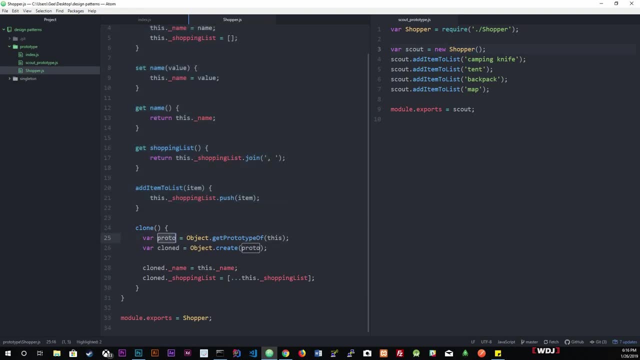 the scout has and just ape posición the scout and peppyOODs and peppys, Asian quería space and player, which is over here. when we clone it, we want to be using the same class the scout has, and just it, or add it to WD, WDJ, Okay, So this is what we're doing right here. Proto is grabbing the. 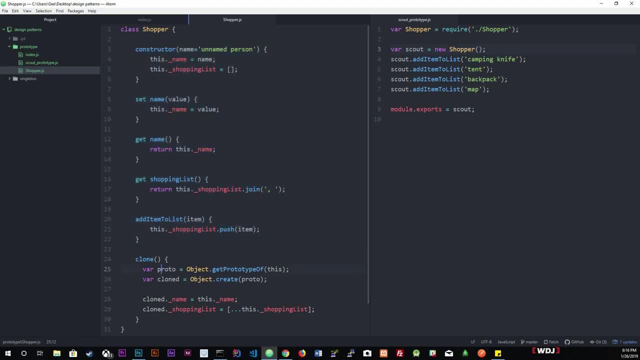 structure the class. and just, we're just right now, we're just grabbing the class, right here We're just grabbing the class. So this one, you could, instead of saying proto, you could literally just say um shopper class copy. We could literally just say it like that: 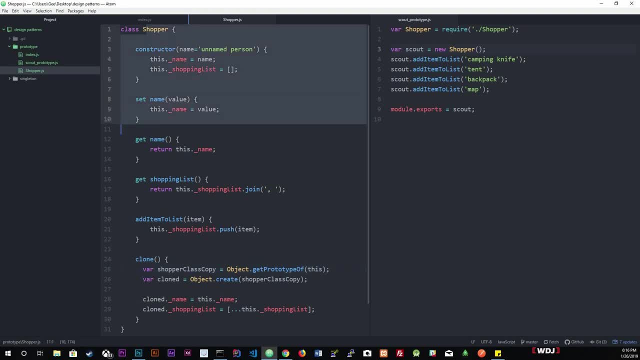 because this right here is literally copying the shopper class, Okay, And down here I'm going to say, uh, instance instead of clone, So that way we can have a better representation. So this instance is: we're going to be creating an instance of this shopper class copy, Okay, And now we're just 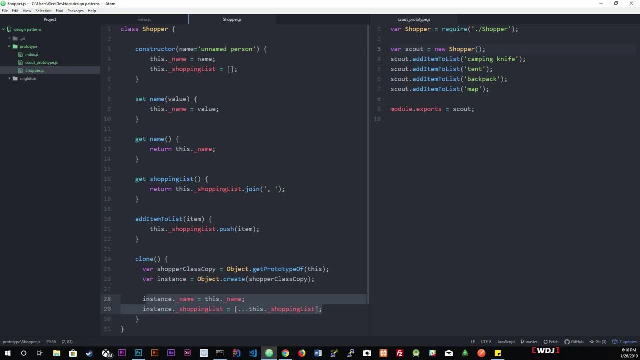 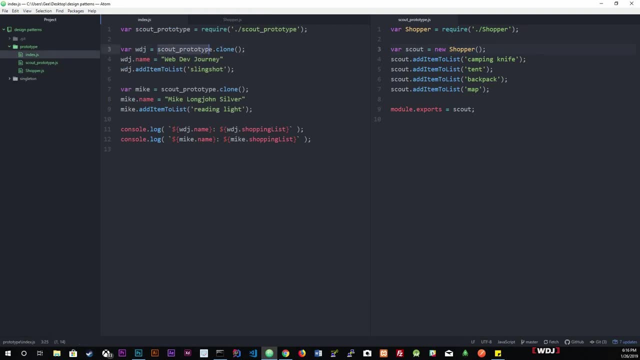 down here, uh, is pretty self-explanatory, but up here is where we're confusing people. I'm pretty sure I'm losing people over here. So over here we just want to be grabbing the scouts class, whatever the scout class is using, or whatever class the scout is using. 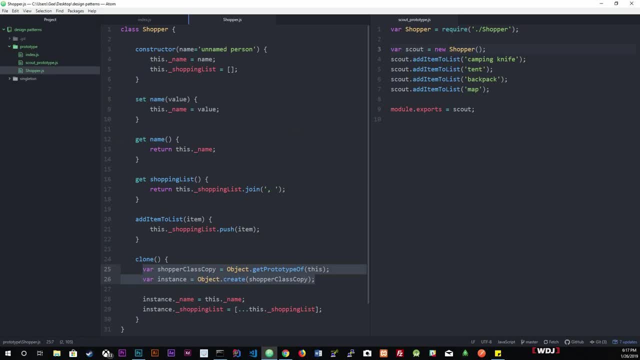 That's what we want to add to WDJ, which is this: right here, We want to grab the scouts class, Okay, Which is this? And now we want to append it to WDJ. This is the instance. WDJ is the instance, Okay, We want to append it, that class to the instance. So that way we have. 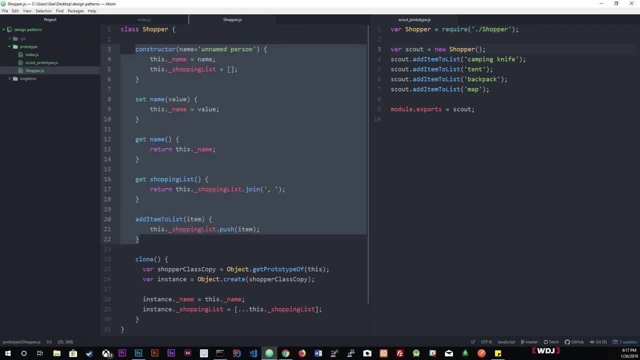 all of these methods added to WDJ. And now we're down here, we're just going to add the scouts class And then we're just adding the name and shopping list. I hope this actually explains a little bit more on why or how this is actually working. but you know for that, guys, we're going to move on to. 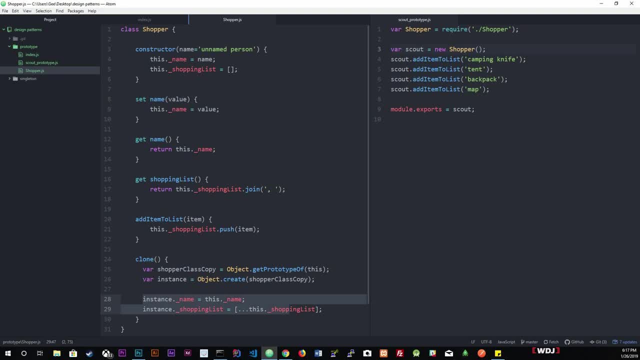 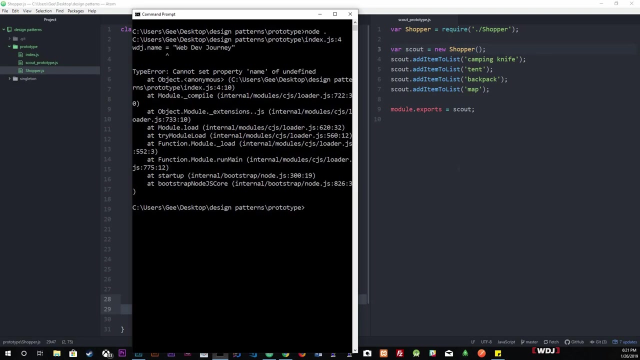 the pros and cons of this actual pattern and where would you actually use it? Um, I'm just, I'm just thinking that I did not run it, So let's run this thing, So that way you can see what's going on and we get a thing. Let me. 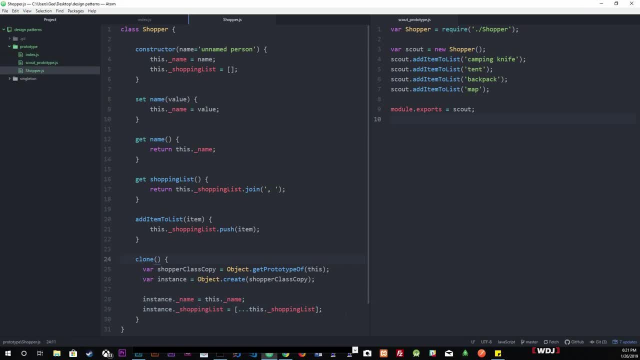 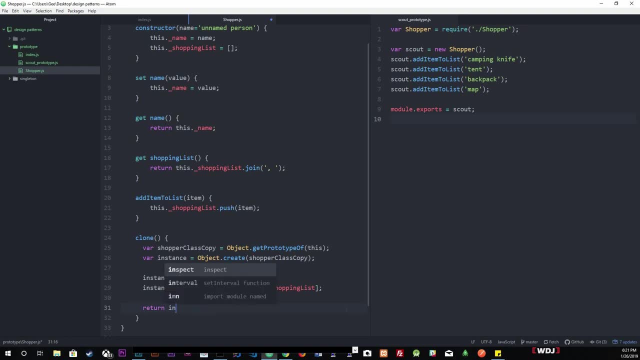 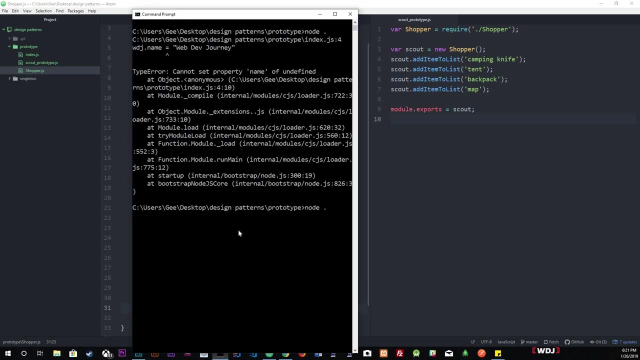 let me fix that real quick. Oh, that's because right here in clone we're not returning the instance. Uh, we need to return it, Instance. Okay, And now, if you run it one more time, you should get it All right. See, uh, web dev has camping, camping knife tent backpack map. 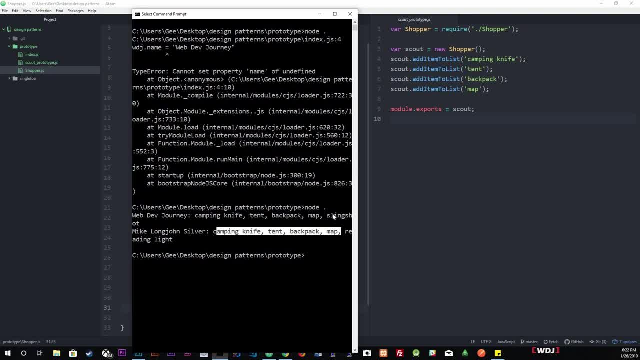 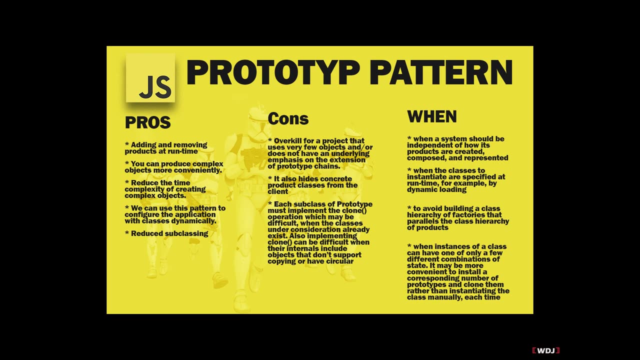 So does, uh, Mike Long and John Silver, And the only difference is web dev has slingshot, while Mike has a reading light, crazy migrating light, Don't know why. but anyways, let's go to the pros and cons and why. So, guys, I do want you to know that the main advantage of this pattern 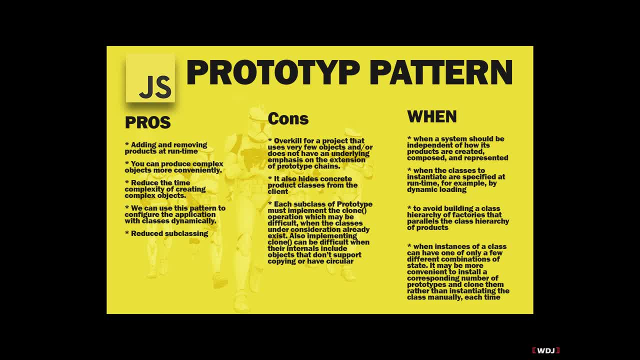 is to have minimal instance creation, um, which might be more costly than actually cloning the instance instead. But let's go on. let's go on to uh pros and cons. The one of the pros is adding and removing products at runtime. uh prototype that you incorporate in new concrete. 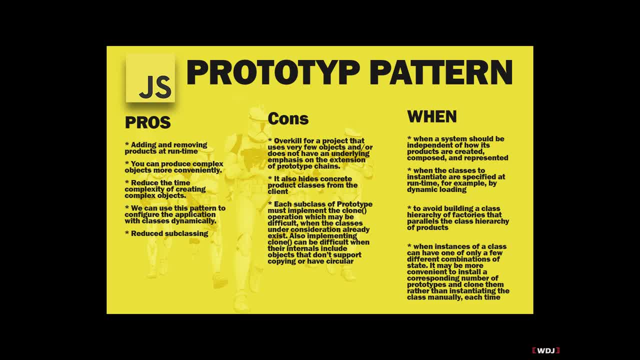 product Class into a system simply by registering a prototypical instance with the client. Now, this is a bit more flexible than other creational patterns, because a client can install and remove prototypes at runtime, And by I mean by other creational patterns is one of them. 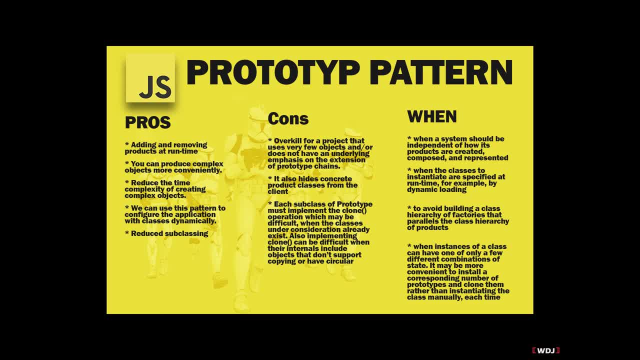 uh, for example, is the factory method, uh, which is going to be in the next video, guys. So you know, stay tuned for that. Another pro is you can produce complex objects more conveniently. Um, like we saw right now. 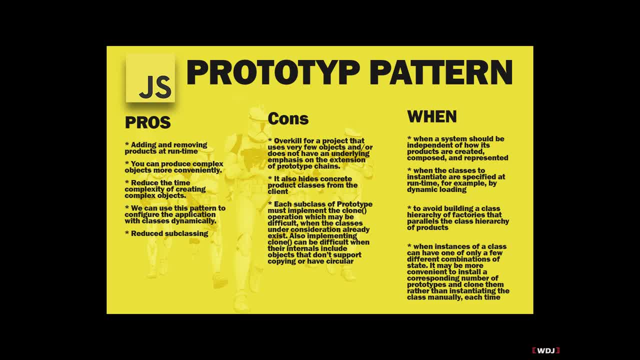 even though my wasn't that complex. but just imagine that you you're dealing with the complex object. Another one is reduce the time complexity of creating complex objects. Now, this ties into the second one that I just said. um, yeah, So if it's a complex object, yes, you're gonna have a hard. 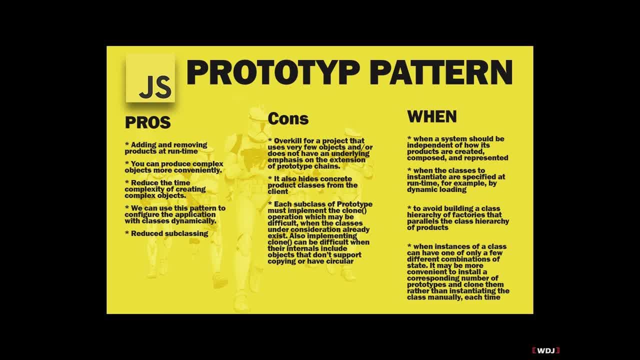 time replicating that instance, Um. and as for the second one, you, you're not going to waste that many resources of your company, your resource and time from your company, so that's a good thing. um, we can use this pattern to configure the application with classes dynamically. 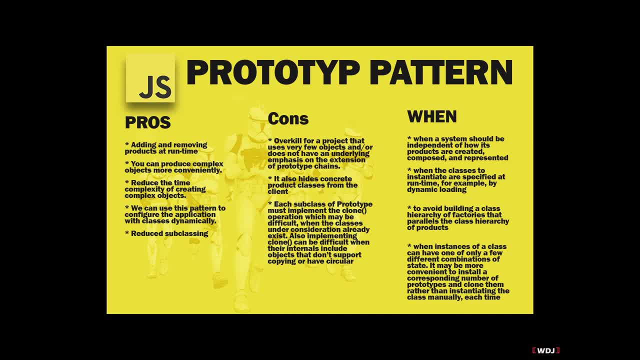 that's pretty self-explanatory. and reduced subclassing, which the factory method, like i said, next video. don't worry, the factory method often produces a hierarchy of creator classes that parallels the product class hierarchy. all right, the prototype pattern lets you clone the prototype instead of asking a factory method to make a new object. 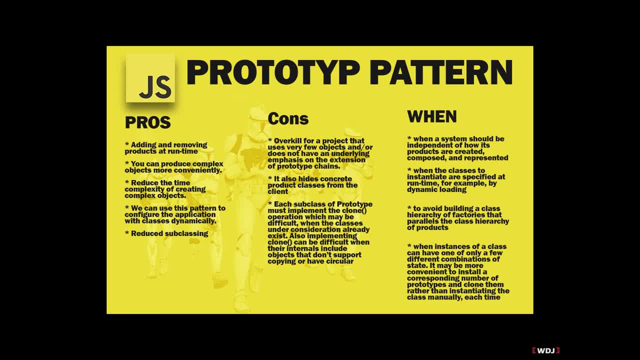 hence you don't need a creator class hierarchy at all. so, moving on to the cons- overkill for, okay, this first one isn't really a- uh, a con, i would say it's just more of a, i guess, letting you know it's an overkill for a project that uses very few objects and 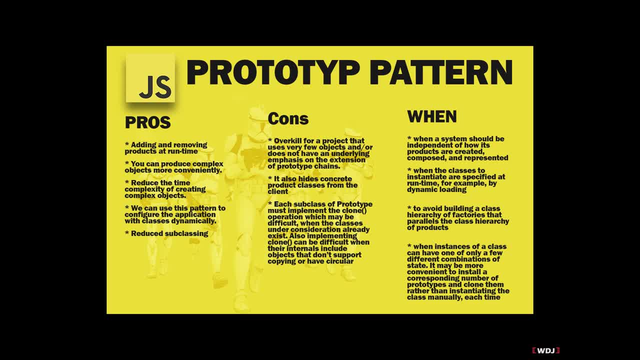 overs Johns口 selbst identificationogen der notch and is not addressable in file complicado or does not have an underlying emphasis of the extension of prototype chains. It also hides concrete product classes from the client and each subclass of prototype must implement the clone operation. 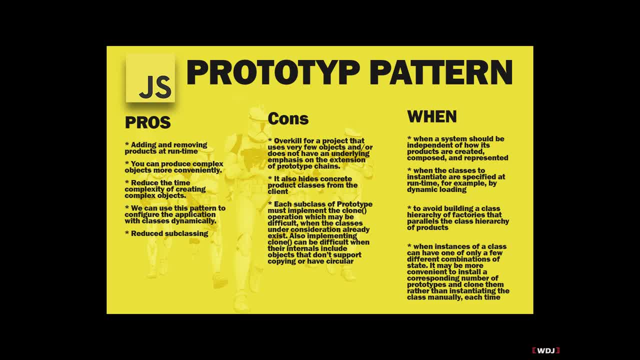 which may be difficult when the classes under consideration already exist. Also, implementing clone can be difficult when their internals include objects that don't support copying or have circular references. I forgot to put references, but, yeah, circular references. When should you use these? 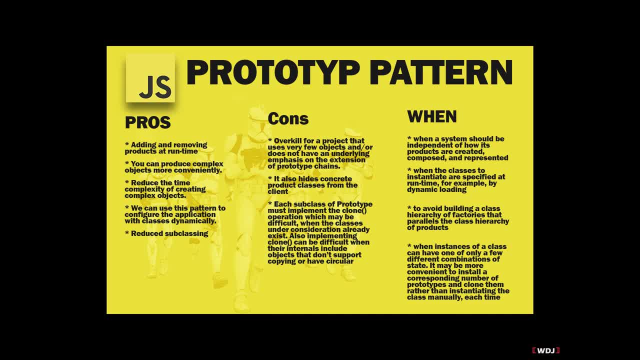 Well, honestly, the Gang of Four actually tell us when, or according to the Gang of Four, this is when you should use them. all right. When a system should be independent of how its products are created, composed and represented. When the classes to instantiate are specified at runtime. 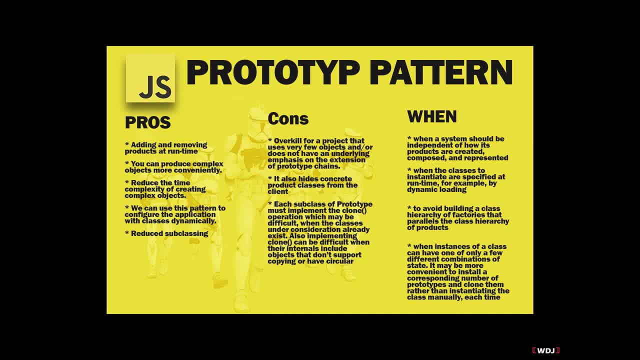 for example by dynamic loading, To avoid building a class hierarchy of factories that parallels the class hierarchy of products, the factory method, When instances of a class can have one of only a few different combinations of state, like the one we did right now. 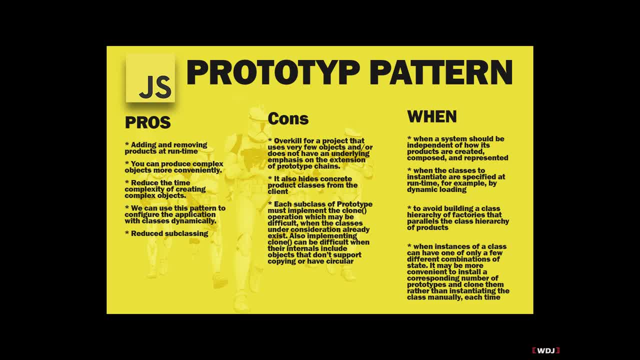 where it only had literally one. we just added one thing to it. that's it. It may be more convenient to install a corresponding number of prototypes and clone them, rather than instantiating the class manually each time we use it. It's just a matter of creating a stateful instance. 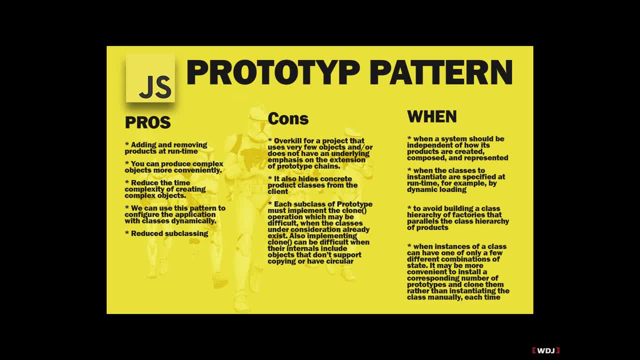 that is consistent with the appropriate state. Now, in my opinion, these are what the Gang of Four tell us that we probably should use a prototype with- But, in my opinion, most common cases where creating a stateful instance is way more expensive than copying an existing instance. 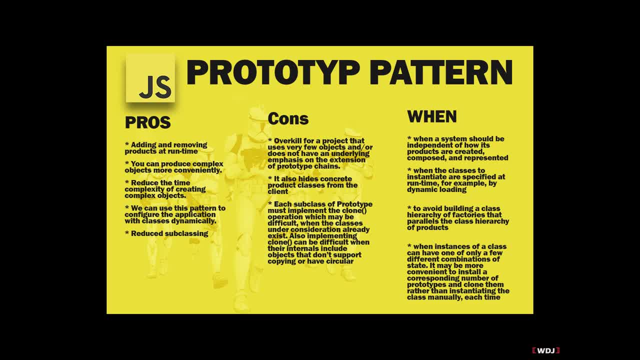 And you need to create lots of this object, Like, for example, if the creation needs to get data from a database connection, get data from the system with system cars or the file system, get data from another server with sockets, web services or whatever- compute a large amount of data. 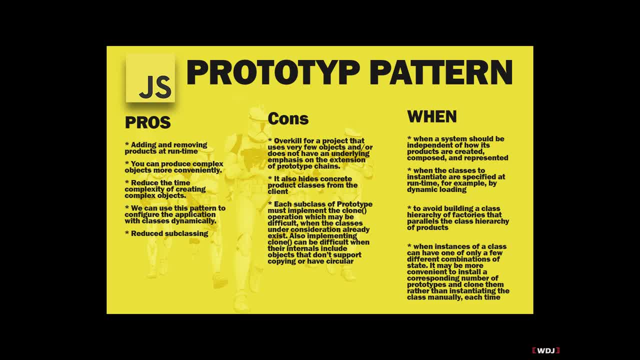 For example, if it needs to sort data, basically anything that takes time, all right. The object must be stateful, because if it has no state, then you should probably be using a singleton. In my previous video, you should probably be using a singleton for that. 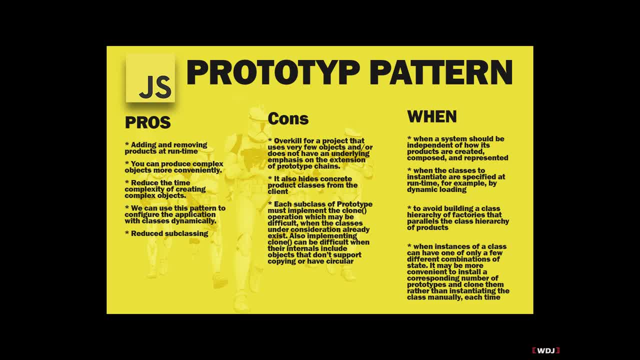 Now there is another use case. if you have an instance that is mutable and you want to give it to another part of the code, for security reasons you might want to give a duplicate instead of the real instance, because the instance can be modified by the client code.